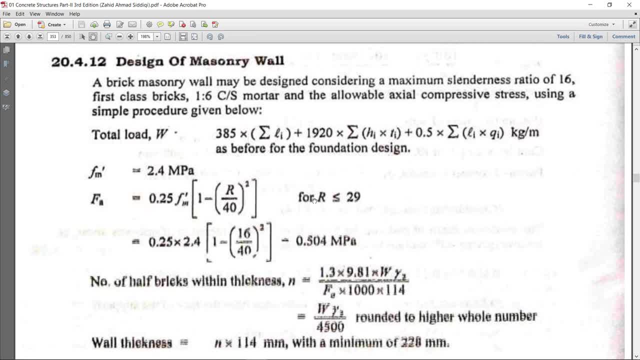 slenderness ratio of the brick. This formula will be used if the slenderness ratio is less than or equal to 29.. Now two things comes in our mind: What is slenderness ratio and why 16 slenderness and why 1 ratio, 6 cement sand mortar is used. So I will go further in the theory. 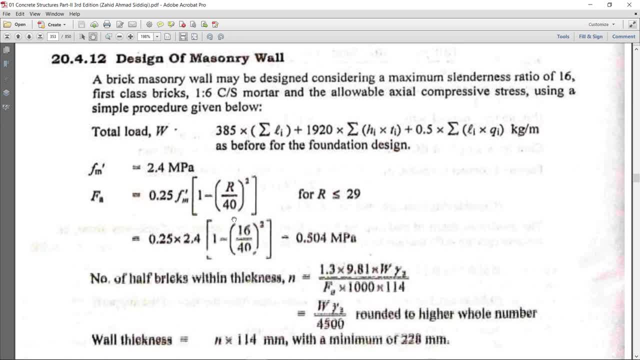 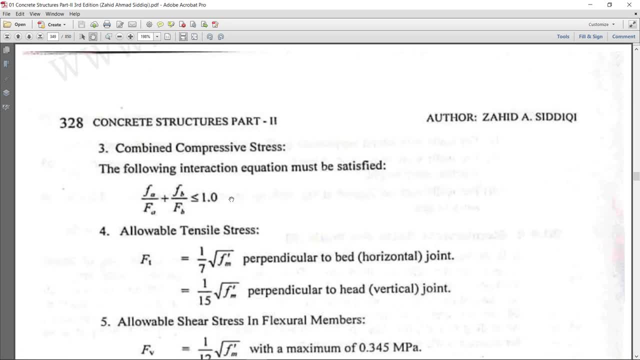 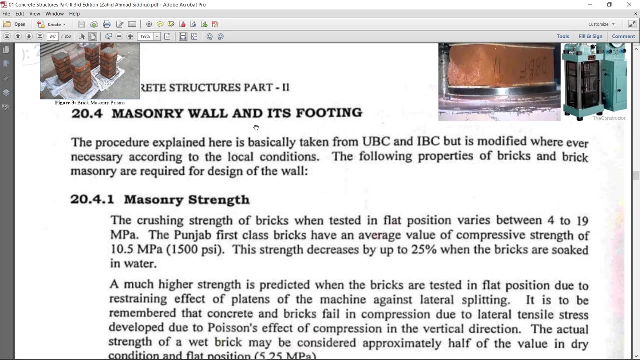 so that I come to some point for the discussion: why the r and slenderness ratio, or what is slenderness ratio, is for the brick wall. Here is the masonry wall and its footing design. The procedure here is discussed, So let's start with the masonry wall First of all. I will 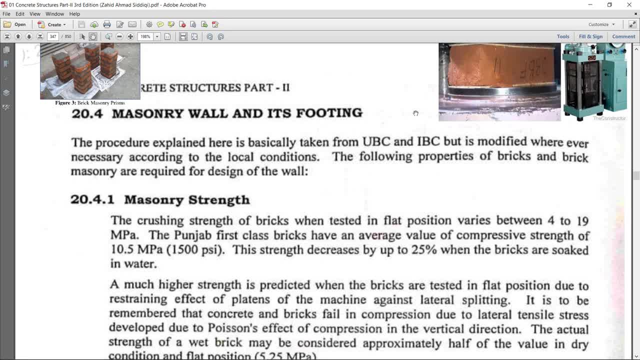 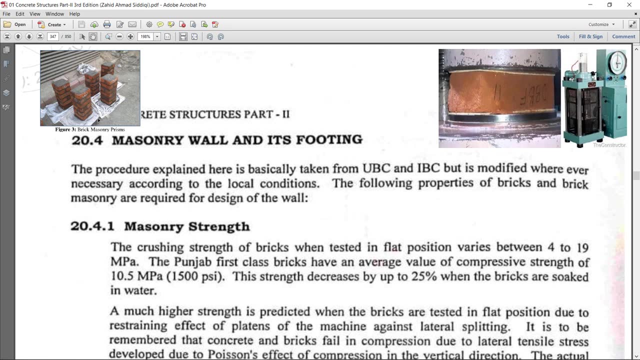 just brief. what is masonry strength and the brick strength? in the brick strength we perform a test on one unit of brick and place in the UTM, you know universal testing machine, and we get the strength of one brick and the masonry strength. that is, we make a unit of bricks. just like courses. 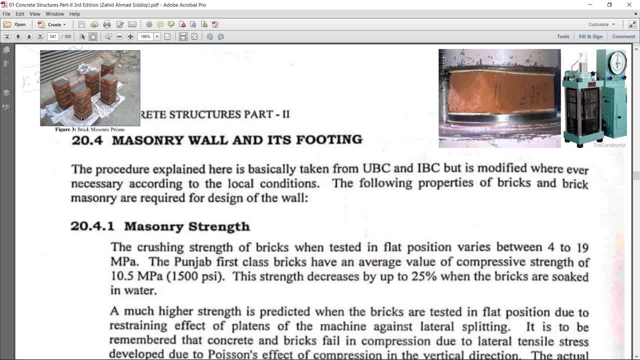 on the one side header face, on the other side stretcher face. we make a masonry unit as per code and and perform the test on this mastery unit. in the UTM the strength of this masonry unit is called masonry strength, so that's the difference between strength of a brick and 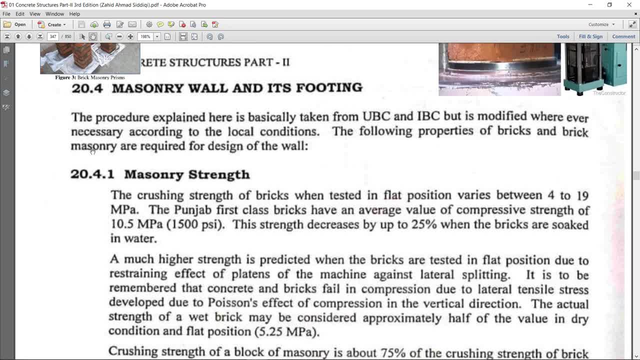 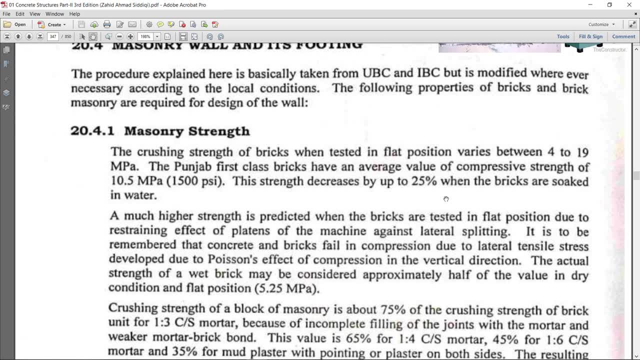 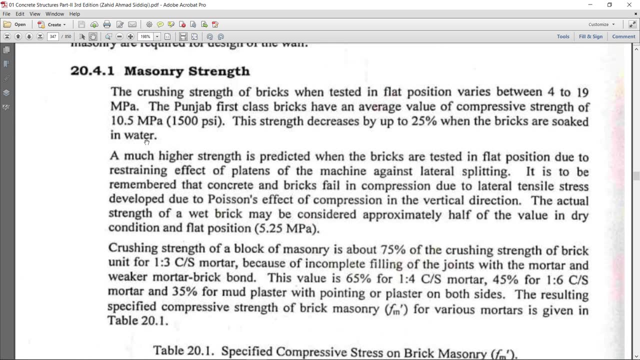 strength of the mastery. so the strength of mastery for the first-class breaks, that is 10 point 5 mega Pascal. but that is 10 point 5 mega Pascal. but that is reduced 25 percent when the bricks are wet means soaked in water. so there is again some theory, uh. 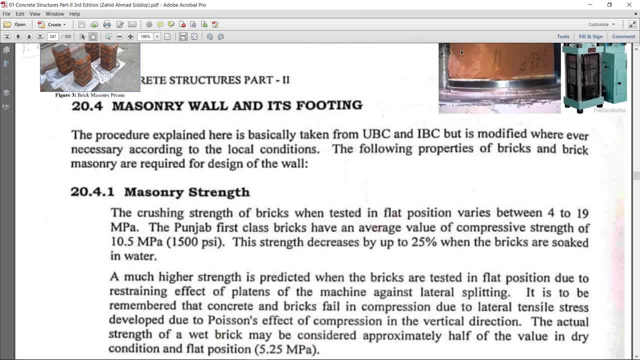 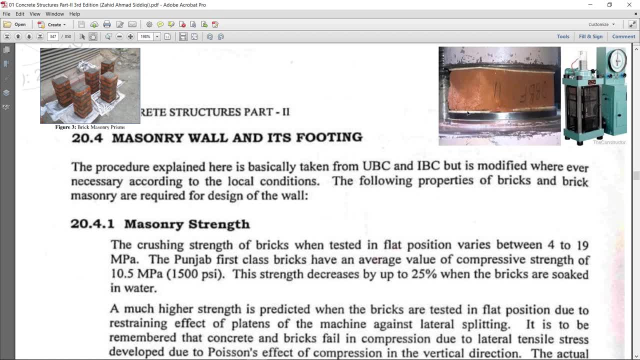 the strength that we get in the utm due to uh, for due to first class break, that strength is much more uh than its actual y duty. due to the end platen effect, due to the ends mean from the uh upper jaws and lower jaws effect. this londoners ratio of this small brick that is less. 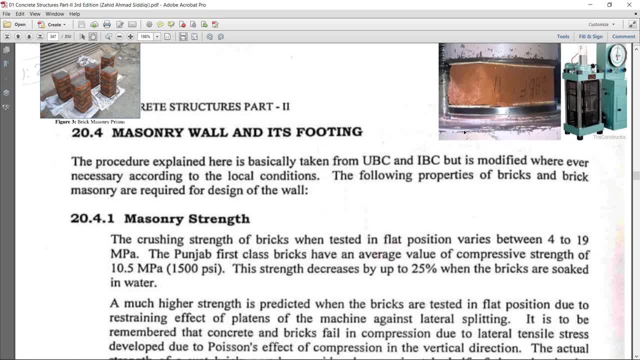 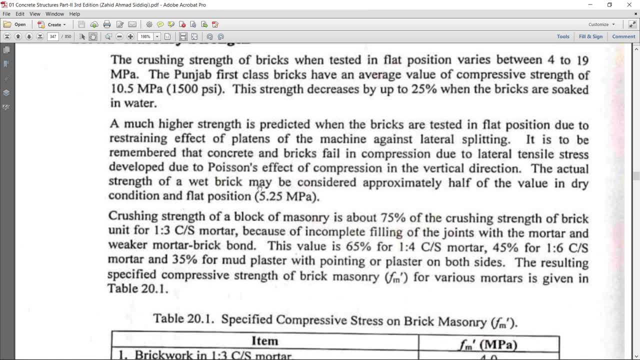 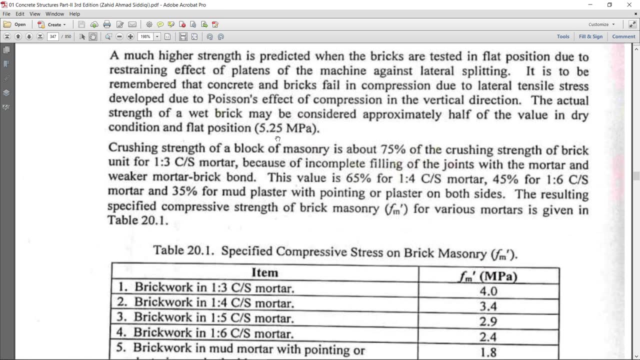 so that's why it strength, we get more. so the author is recommended that instead of using this strength of brick 10.5, we will use half of the strength, just like 5.25 megapascal. so this is the strength of one brick. so when we test in the masonry unit, 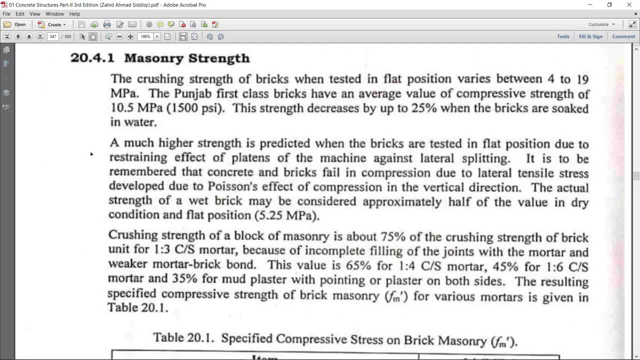 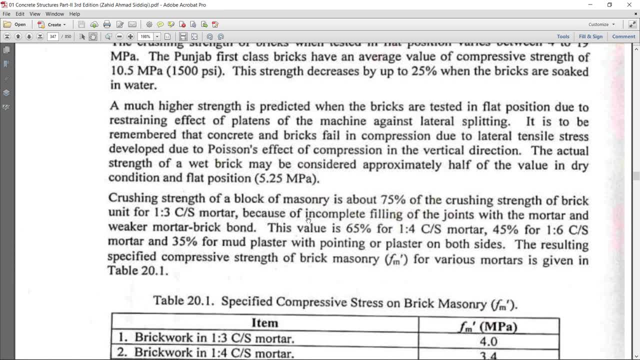 the bricks, first class bricks with mortar. the crushing strength of block masonry is about 75 percent of the crushing strength of the brick. when we use one ratio three, cement sand mortar, and it is 65 percent. when we use one ratio four, cement sand, it is 45 percent. uh, one ratio six, cement sand mortar. 35. 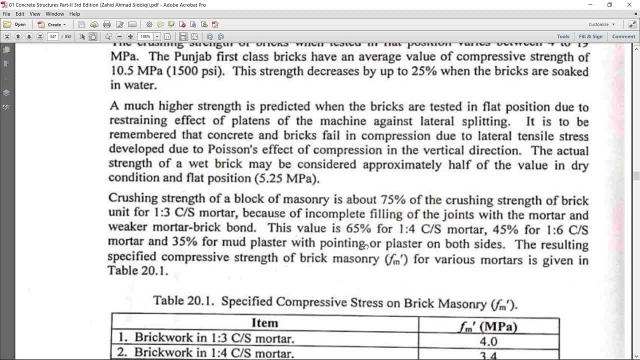 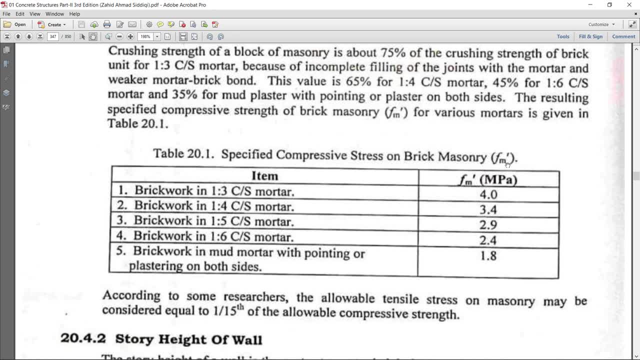 percent when we use mud plaster with pointing or plaster on both sides. so the brick masonry strength, that is fm dash in one ratio three. cement sand mortar, that is four, one ratio four, 3.4. when in the fifth brick work in mud mortar means the jointing of the bricks are 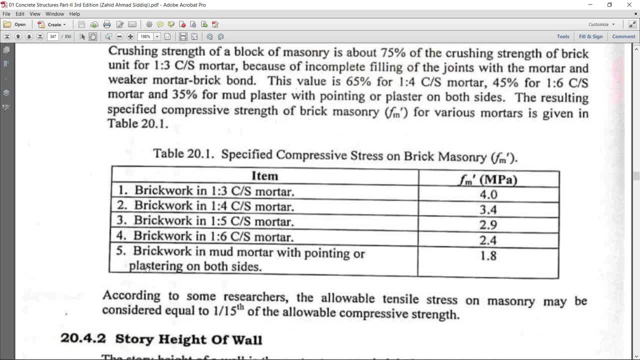 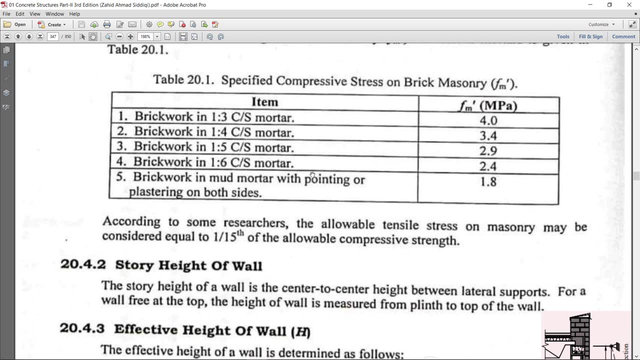 done with the mud and on the outside of the wall the plaster is present. plaster is present, then the mastery strength, that is 1.8. so let's first test w and the endless waiting was of 1,8 for brick, for mud and for getting the strength of 1 ratio 3. 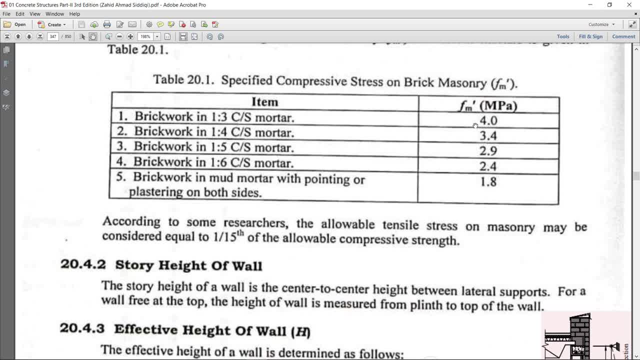 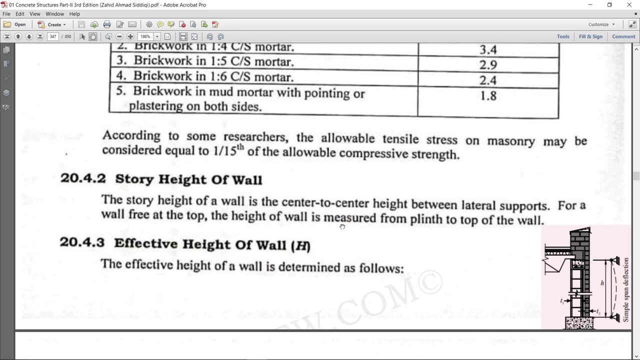 we can take one over 15 into four. we get the tensile strength of break. we almost ignore and do in the design the tensile strength because that is too low now. the second step is story height of the wall. story height of the wall that is, for example, here see, there is a foundation and here is a floor. so the the distance between 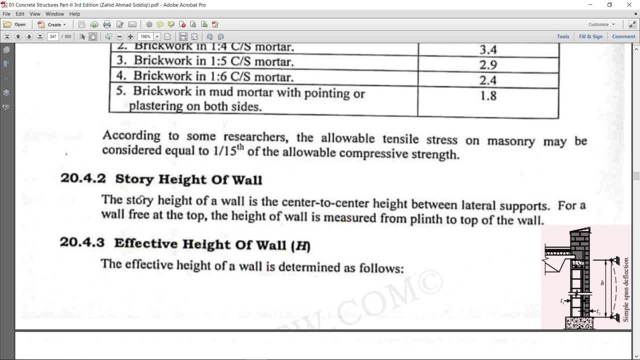 two sports. that is the story height of the wall. the story height of a wall is the center to center height between lateral sport mean the distance from this center of the sport and from the foundation. so that is the story height of the wall. uh, for a wall free at top, the height of wall is: 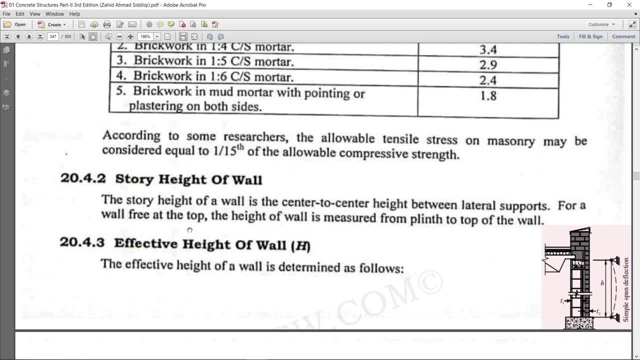 measured from the plinth to the top of the wall, because at top there is no sport, so no need to take from center, so we will take from the foundation to the top of the wall. now that is a new thing. that is the effective height of wall that we use to measure the height of the wall. 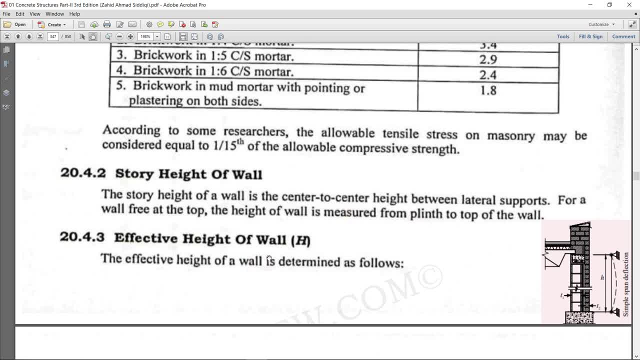 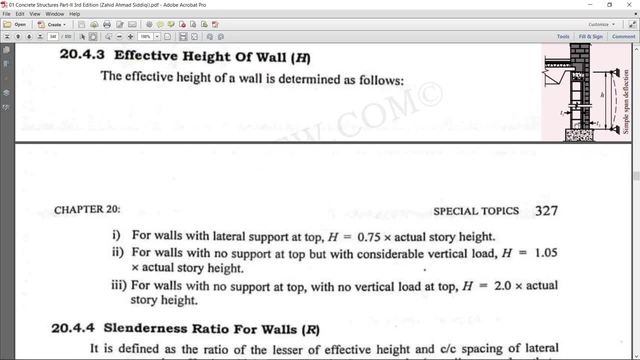 using the design. so what is the effective height of the wall? there are three conditions for wall: with lateral sport at top. here you can see this wall has sport at the top due to the slab or due to joy slab whatsoever. there is a sport at top and sport at bottom. so we will get the 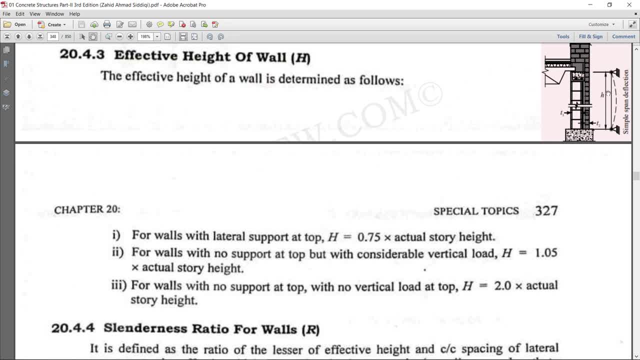 effective height whatsoever. the actual height, for example. the actual height is h. we will multiply with 0.5 and get the height of a effective height of the wall. this is the first condition for walls with no sport at top but with a considerable vertical height. h effective height will be 1.05 to the actual height. 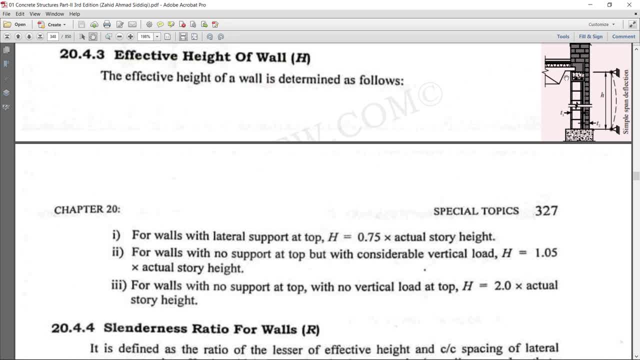 means if there is a no sport at top, uh, then there, uh, no sport at top, but there is a vertical. vertical load is present, but no, there is no sport. uh, for then the effective height, that is 1.05 of actual height. the third condition: there is no sport at the top, but also 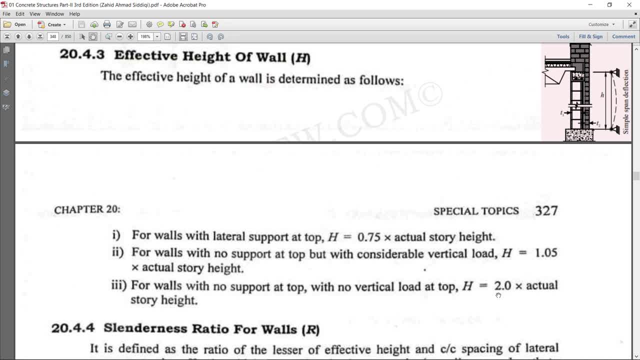 there is no vertical load at top, then the effective height will be 2 times the actual height. that is the effective height, then the effective width of the wall or effective thickness of the wall. so that is the uh outer dimensions of the wall. so for example, without plaster, the nine inch wall has the effective 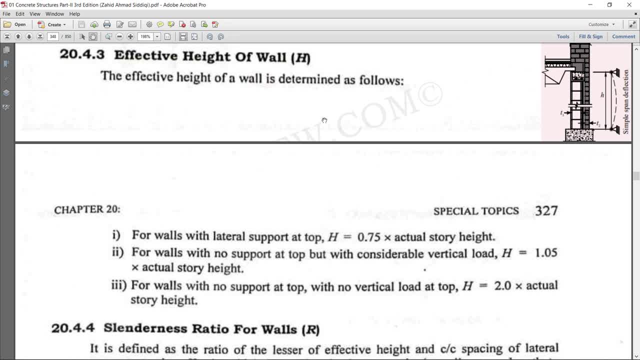 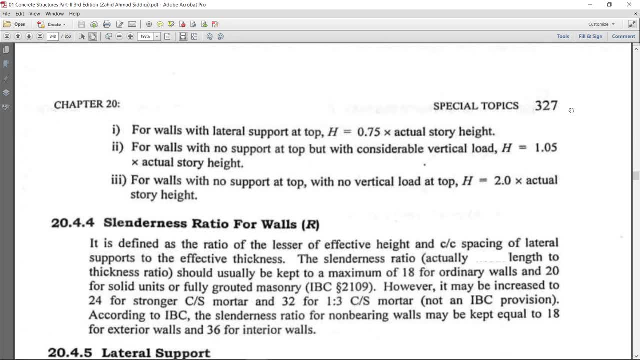 height nine inch. so that's how we take the effective width, that is the effective height, and there is another that is effective thickness or effective width. now, what is slenderness ratio? it is the ratio of length to thickness. it is defined as the ratio of lesser of effective height. 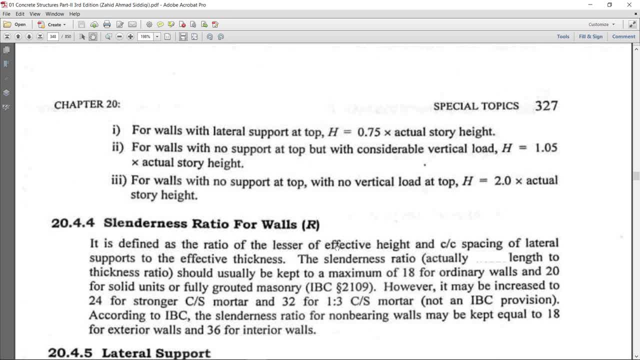 and center of center spacing of lateral sport. in simple words, to the effective thickness. the slenderness ratio actually is length to thickness ratio. that is the simple formula. so in the upper length divided by thickness, length can be either effective height or center to center spacing. we will use lesser of both. 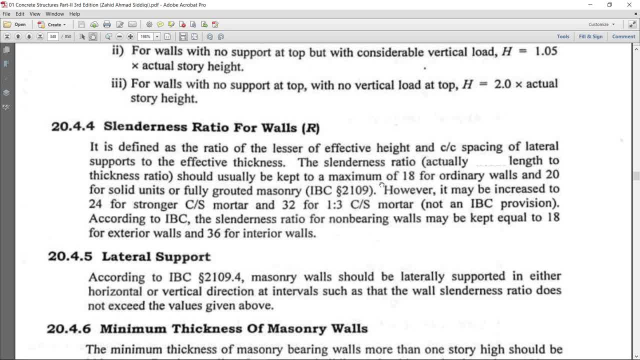 in the formula of slenderness ratio, so it should be not more than 18 for ordinary walls unit or fully grouted masonry unit where a high content of cement is present. However, it may be increased to 24 for stronger cement sand mortar, 32 for one ratio. 3 cement. 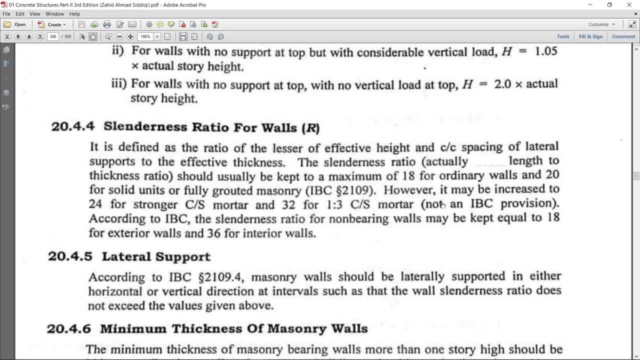 sand mortar. This is the author's provision, author's recommendation, but not the court. According to the IBC International Building Court, the slender ratio for non-beading walls may be kept equal to 18 for exterior walls and 36 for interior walls. 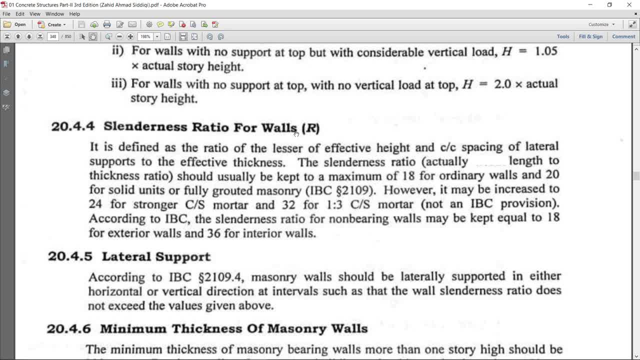 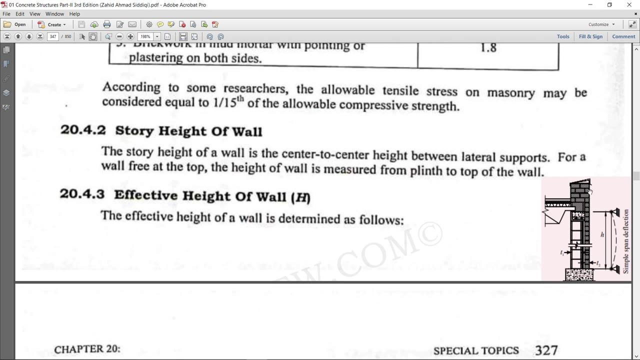 So that is the simple definition of slender. ratio is for walls. The symbol is R, That is the height of the wall divided by the thickness of the wall. So lateral support, Whatsoever the support, Either it is supported by pins or supported by slabs. 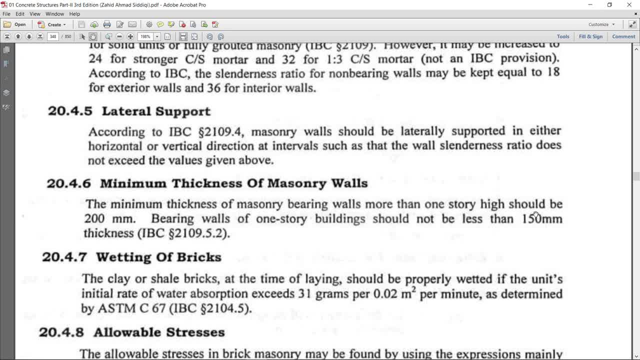 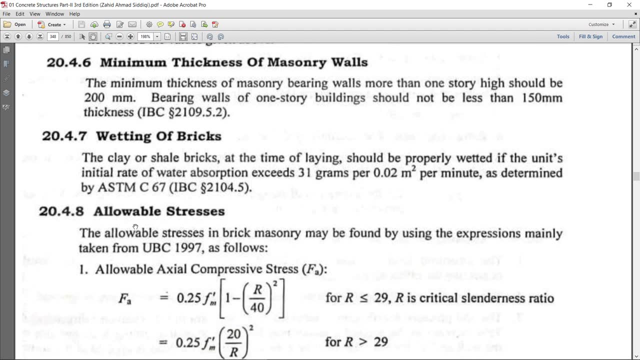 So whatsoever. that are the lateral supports. Minimum thickness for masonry wall: The court has recommended that your minimum thickness for load-beading walls should not be less than 200 millimeter, means should not be less than eight inch. Now wetting of bricks. 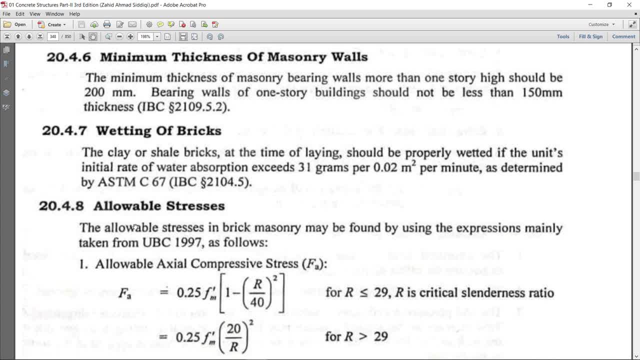 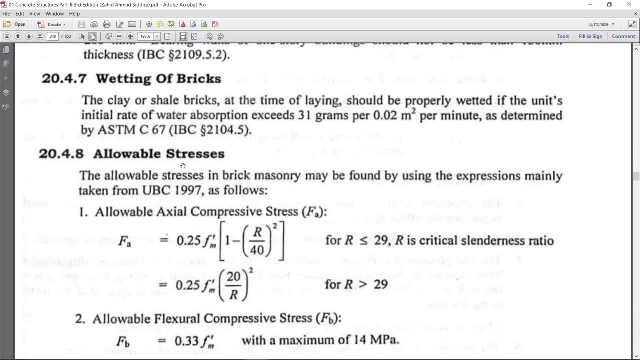 Definitely for doing the coursework of bricks. We Wet the bricks before laying on the walls. Now the next is allowable stresses. So here is, as per UBC, Uniform Building Court, there is a formula given for allowable axial compressive stress That is 0.25 FM. dash, 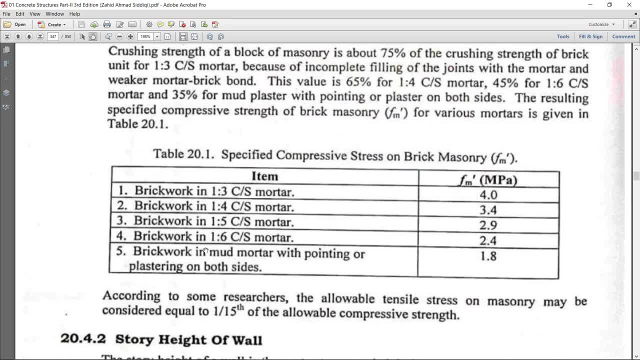 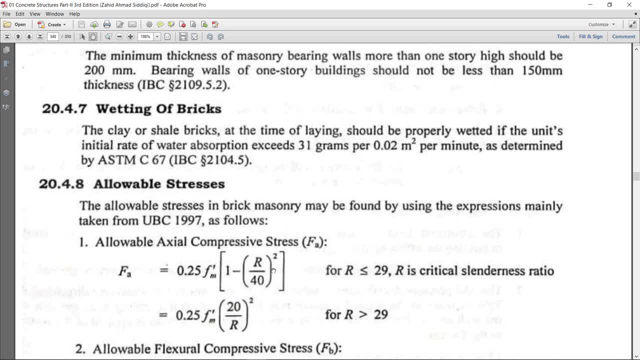 That is a masonry strength That I have shown in this FM. dash Into one minus R over 40 power, whole square. That is a masonry strength That I have shown in this FM. dash Into one minus R over 40 power whole square. 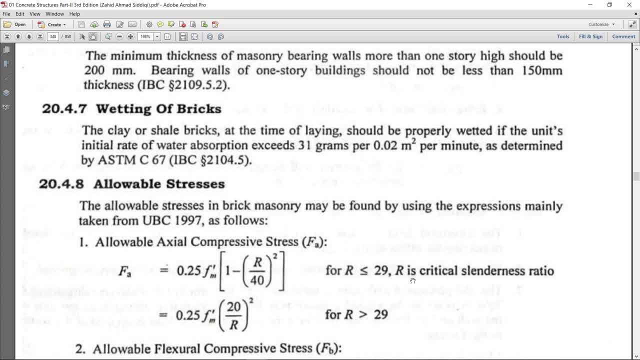 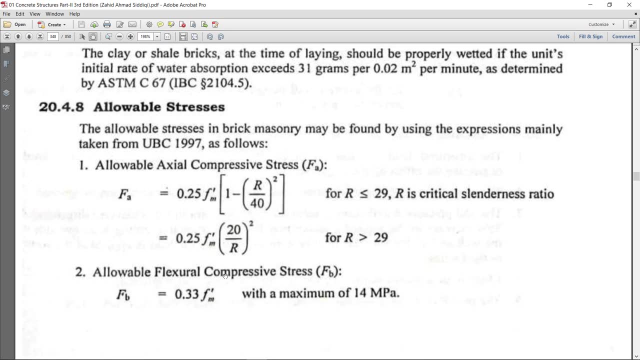 That is a Frieden 70 for slender…. I have shown in this FM dash próximo square: " That is the xl compressive stress of brick Of庩. To get the alliable luxury mean bending compressive stress. That is a 0.33 FM dash. 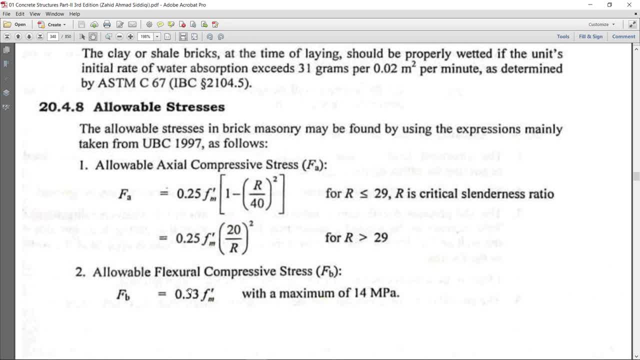 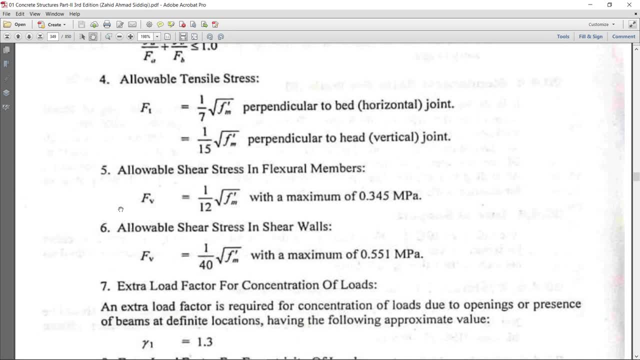 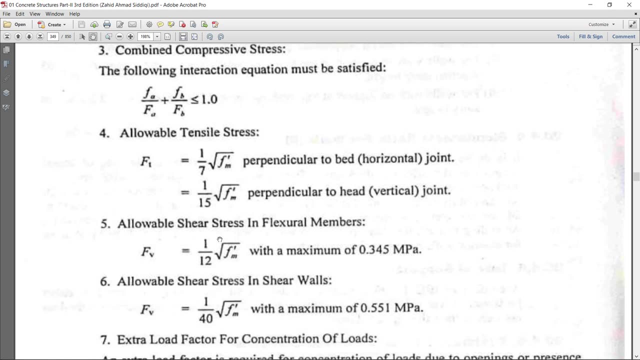 That… Mausoleum in Teăn nodule in print: 0.33 mm. So allowable axial stress- now i will go further, that is again other formulas combined: compressive stress. allowable tensile stress. allowable shear stress, allowable shear stress in shear wall. so 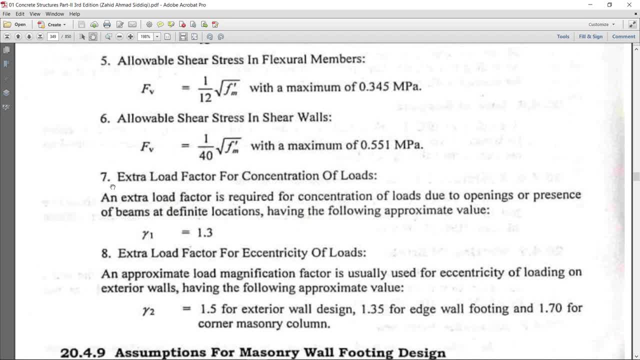 next thing for our design of wall that is important, that is seven and eight point. extra load factor for concentration of floors, extra load factor, for example, if we designing a wall there is some eccentricity like there is no, not the uniform load, why? in our wall mostly? 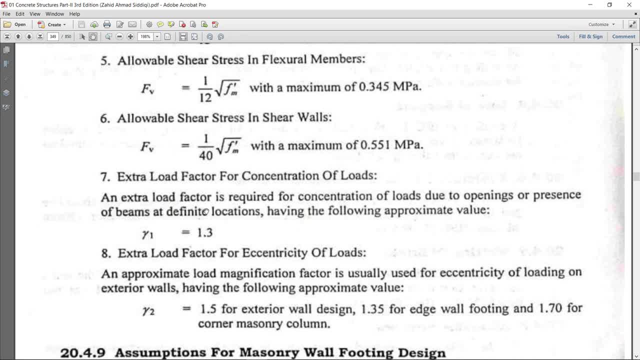 there are openings, like opening due to door, due to windows. so author has recommended that you should. for the designing of wall you should use the factor gamma 1, 1.3. second extra load factor for eccentricity of floor. why when we place the footing it is option that. 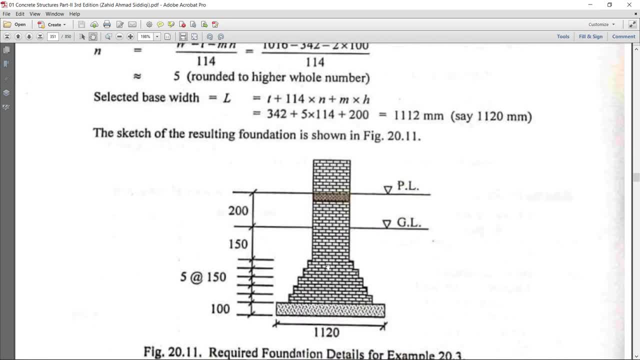 we place the footing on the side of the wall or the side of the wall, and then the steps of the footing may be present on the one side due to the, and not present on this other side by, for example, your exterior walls are attached to the other person or other person neighborhood. 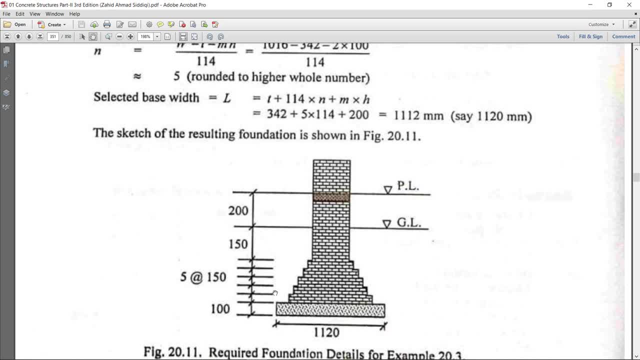 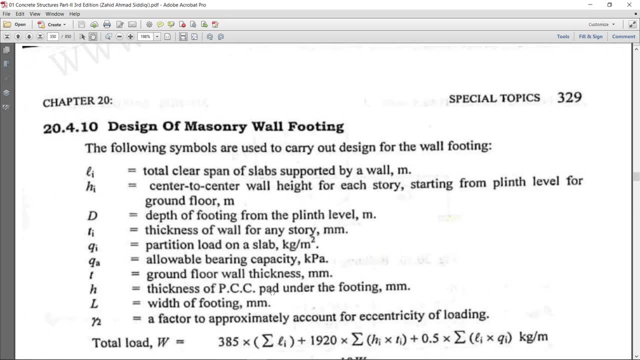 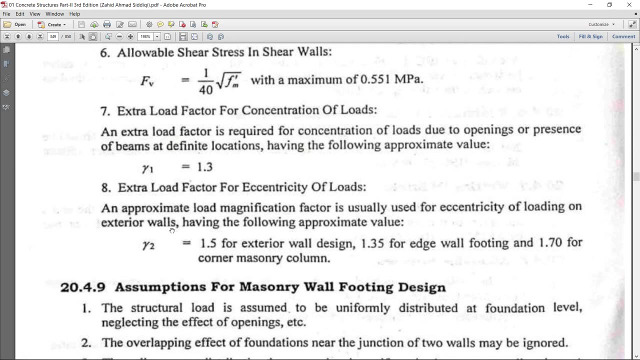 property so you will not be able. your one side of steps on on his property so you have to construct the exterior walls without the steps on the one side. that's the condition you have to again magnify. if your condition is just like that for lower magnification.